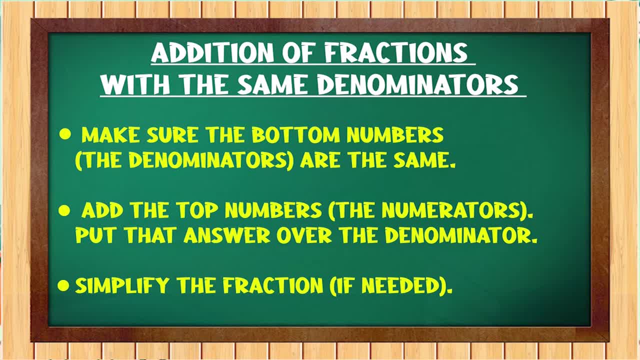 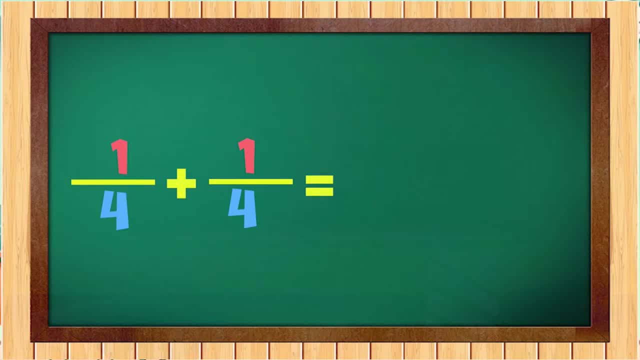 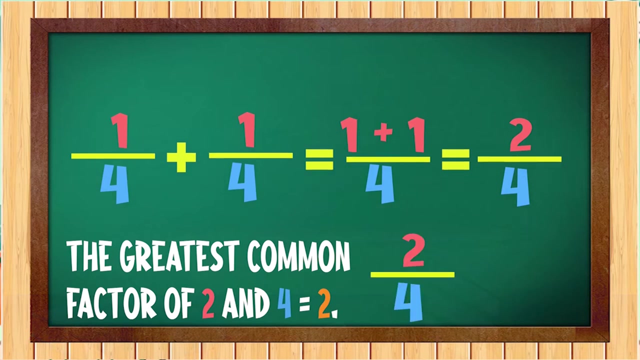 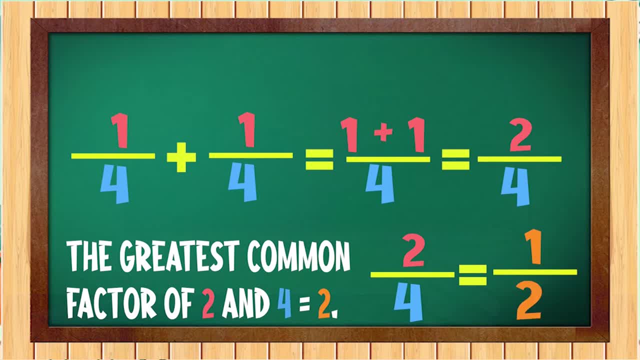 By 4, we'll get 2. So the simplified version of our answer would be half. 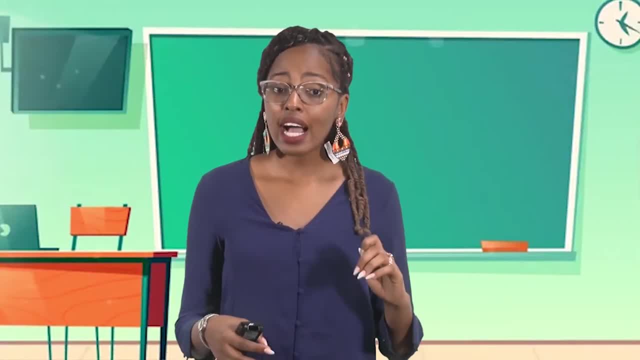 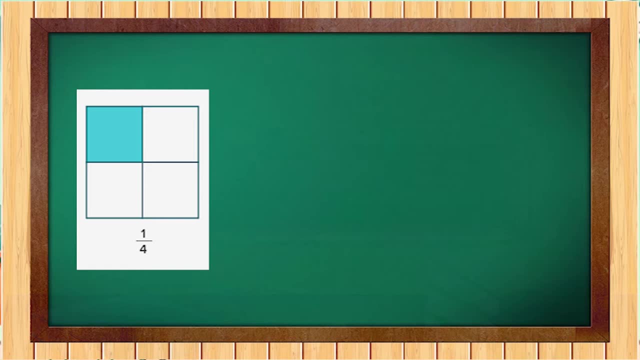 Let's look at it in a picture format. We were asked to find the sum of quarter and quarter. To do this, we're going to look at a square, and we're going to divide that square into 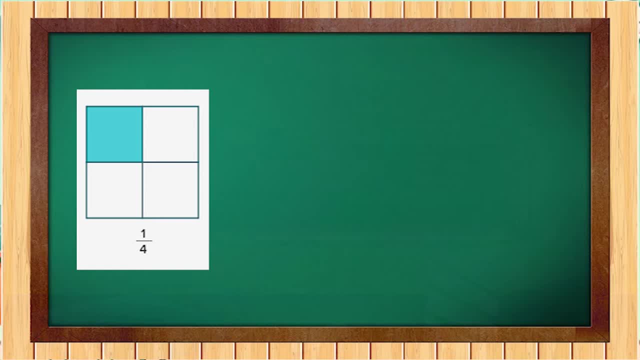 4 equal parts and shade 1 part. And that 1 part that is shaded represents quarter. We do the same for the other one because the fractions are 6. 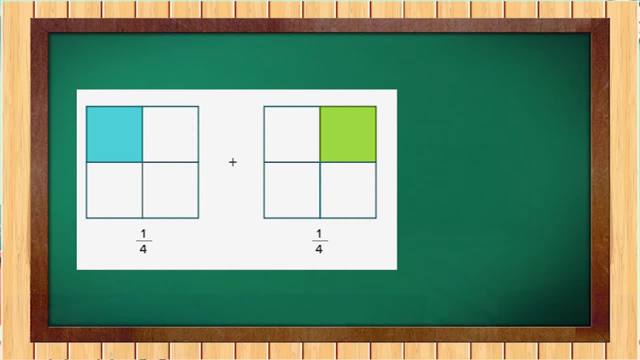 Now, when you add quarter plus quarter, you'll get two quarters, obviously. However, notice that two quarter is similar to half because half of the shape is shaded. 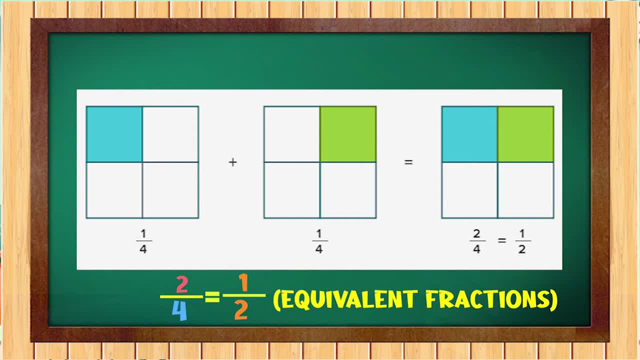 Therefore, two quarters and half are equivalent fractions, meaning they are equal to the same amount. 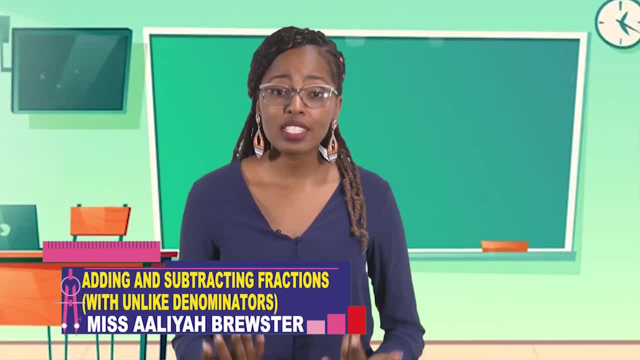 Now that we have an understanding of how to add fractions with similar denominators, 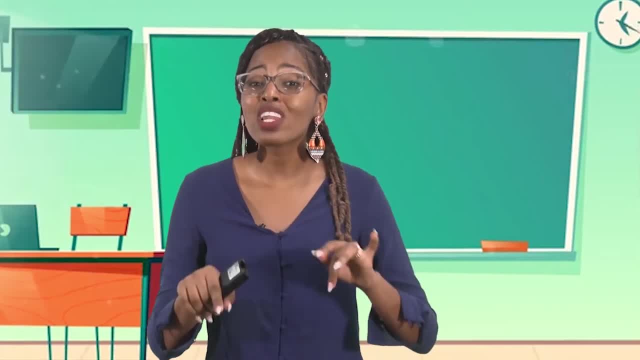 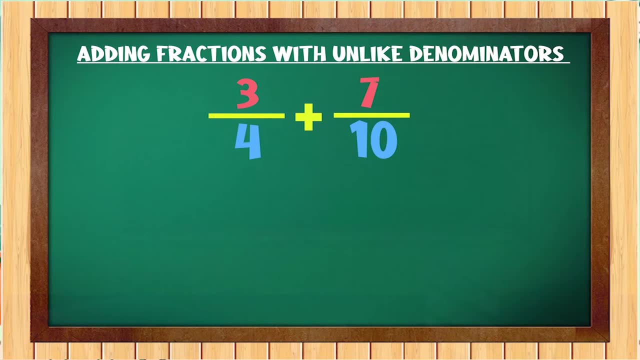 let's look at adding fractions with unlike denominators. In this case, the fractions that we are given, the denominators are not the same. Here we have three quarters plus seven tenths. Notice, for one fraction, the denominator is four. While the other, the denominator is ten. How do we go about solving this? We have to find the LCM of the two denominators. And LCM stands for the lowest common multiple. 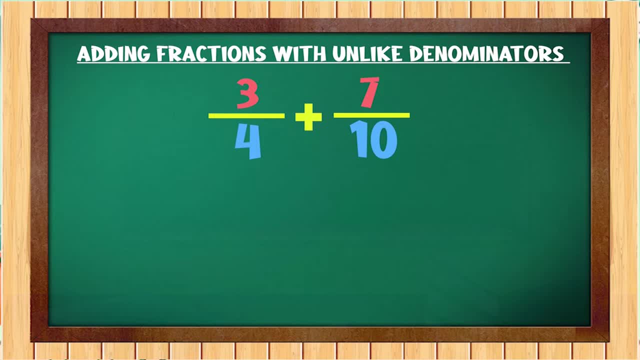 So, if you would like to add the fractions three quarter and seven tenths, 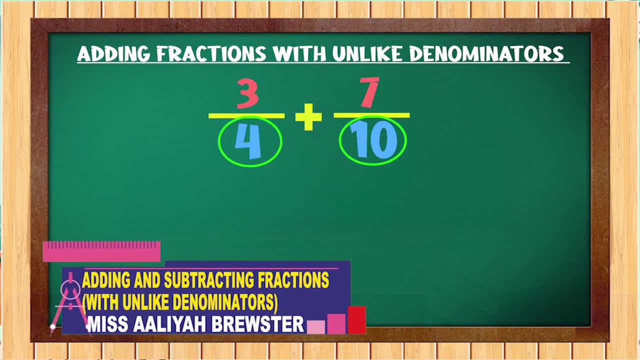 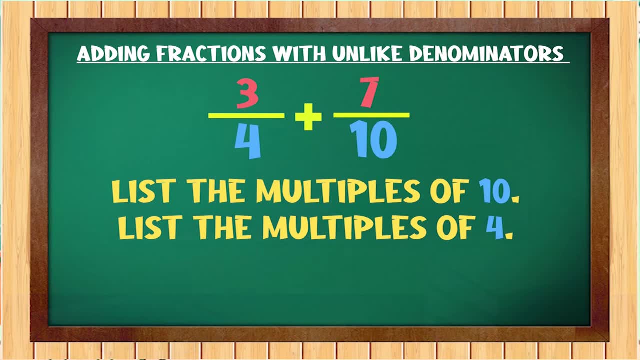 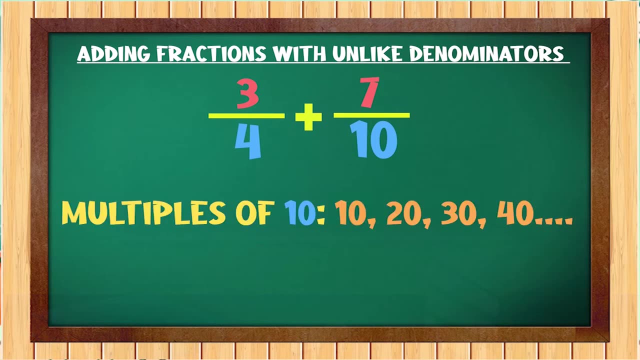 we have to first find the LCM of the two denominators. Here is how we identify the LCM. We have to list the multiples of ten and list the multiples of four. The multiples of ten are ten, twenty, thirty, forty, fifty, sixty. We can go on, but you have to stop at some point. The multiples of four are four, eight, twelve, sixteen, twenty. Now, looking at the multiples of ten and four, we see the lowest common multiple. 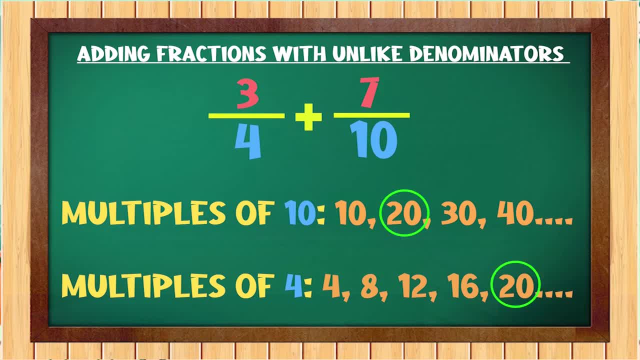 The lowest common multiple is twenty. Or, in other words, four and ten share a similar multiple, which is twenty. Okay? 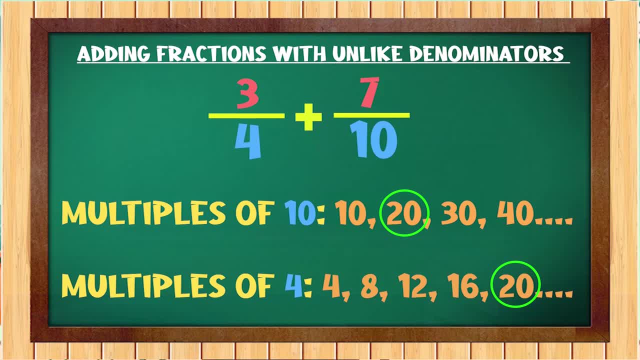 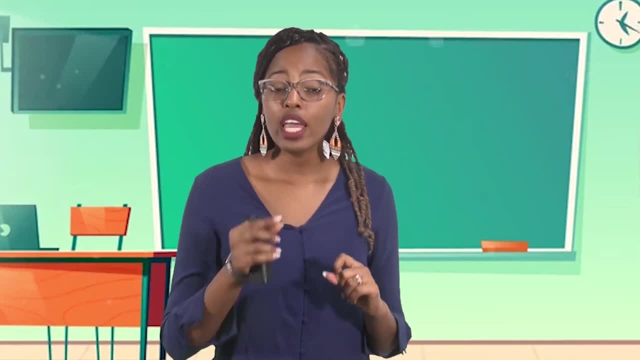 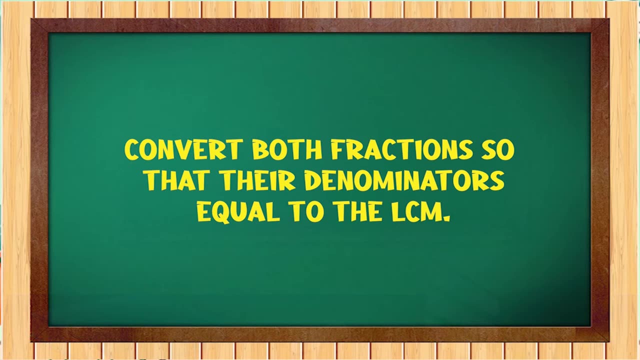 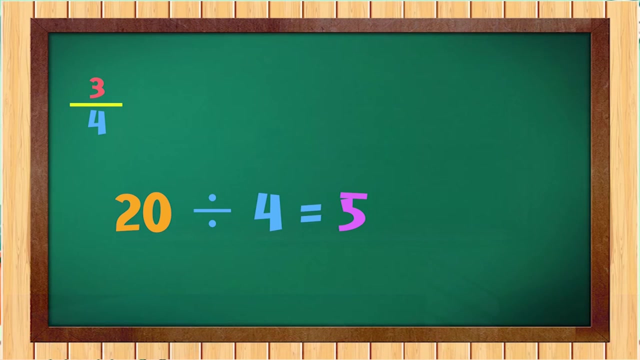 So, we're going to use twenty as our LCM. Continuing with our work in, now that we know the LCM is twenty, we can convert both fractions to make them equal, so that it's easier for us to add. To do this, let's look at the first fraction, which is three quarter. We divide the denominator by the LCM. In this case, twenty divided by four is equivalent to five. Okay? 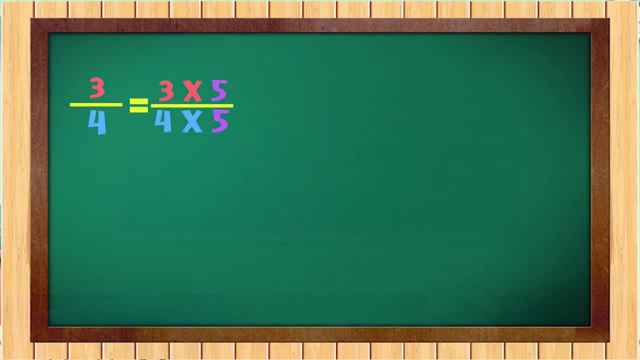 Now, we multiply five by the numerator and five by the denominator. So, five times three is fifteen, and five times four is twenty. So, three quarters is converted. Now, let's look at the second fraction, which is seven tenths. So, we're going to convert this. To do this, we're going to divide the denominator by the LCM. So it's twenty divided by ten. Twenty divided by ten is two. 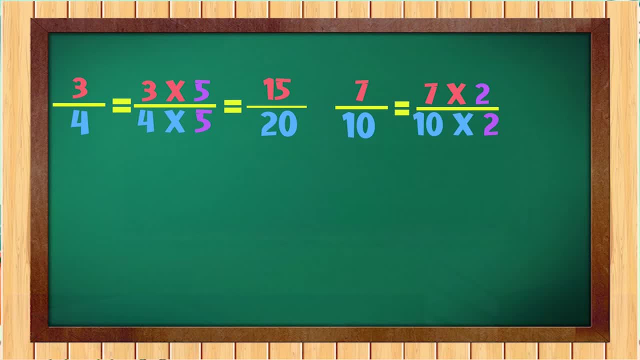 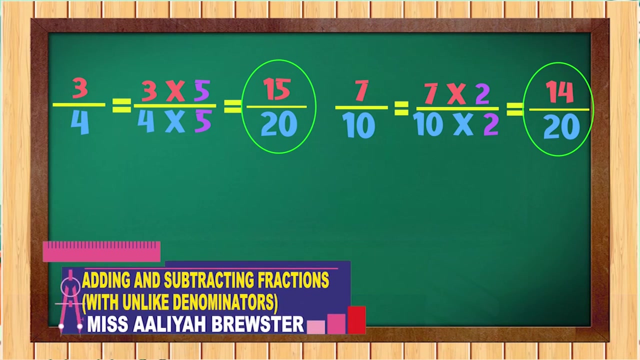 So we multiply two times seven and two times ten. Two times seven is fourteen, while two times ten is twenty. So, seven tenths is converted into fourteen twenties. Now that both fractions are converted, we can substitute those two fractions for the original ones and add. At this point, we have two fractions that have the same denominator, so all we need to do is add the numerator, because the denominator would remain the same in our answer. In this case, our denominator is twenty. So we're going to add fifteen plus fourteen, and that would give us twenty-nine. 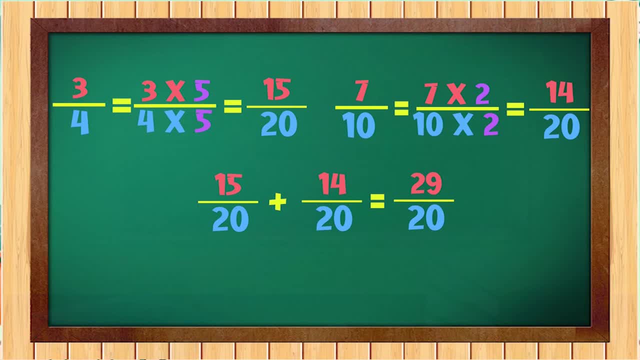 So the answer for our problem is twenty-nine twenties. Well, you would notice that that answer is in the form of an improper fraction. So, we can simplify it by converting it into a mixed number. Remember, boys and girls. 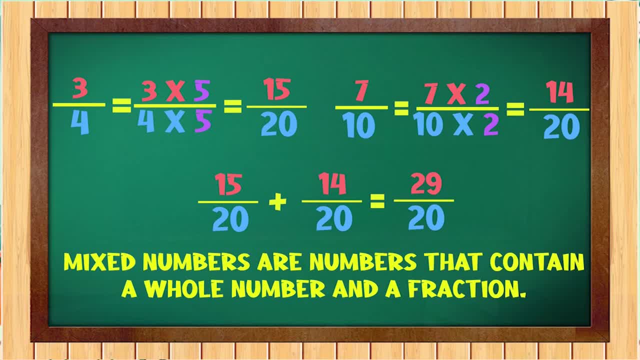 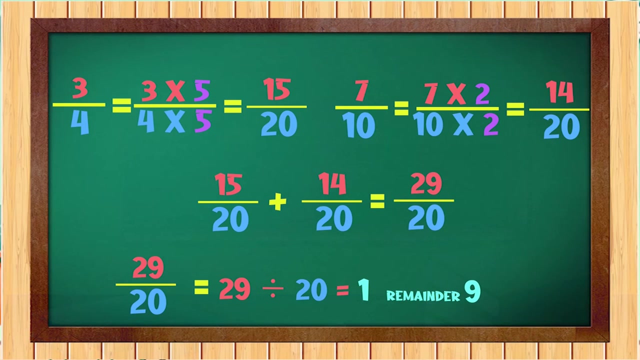 mixed numbers are numbers that contain a whole number and the fraction. To convert the improper fraction into a mixed number, we simply divide the denominator by the numerator and write the remainder as our new numerator. So in this case, we have 29 20s. 20 divided by 29 would give us 1 because 20 can go into 29 one time, but we will have a remainder of 9. So our whole number for the mixed number would be 1 and our new numerator would be 9 and our denominator remains at 20. So our answer then is 1 and 9 20s. Now let's move on to discuss 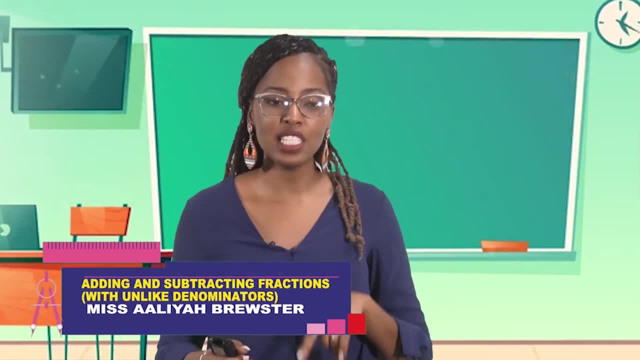 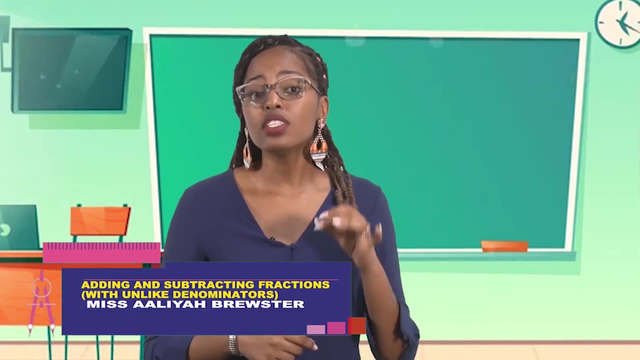 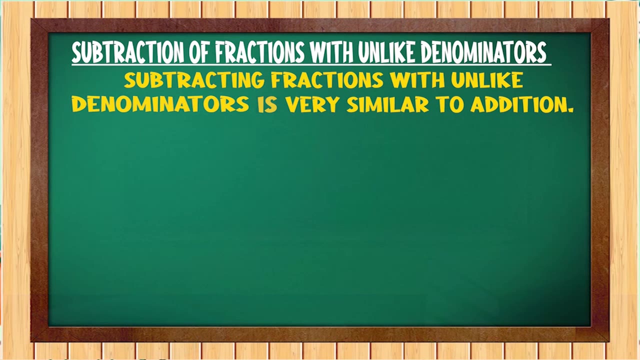 how to convert the improper fraction into a mixed number. So in this case, we have a subtract fraction with unlike denominators. So before we did adding fractions with unlike denominators. Now we're going to subtract. To subtract fractions with unlike denominators, the method of doing it, it's quite similar to adding fractions with unlike denominators. 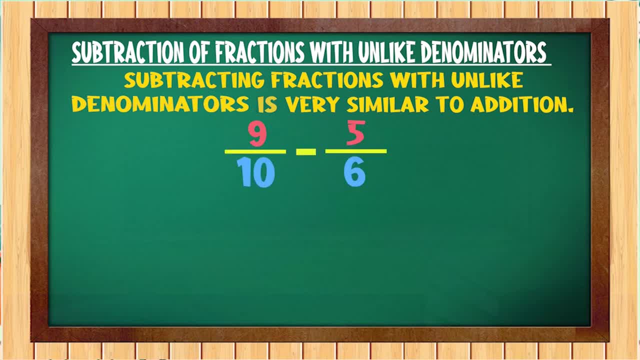 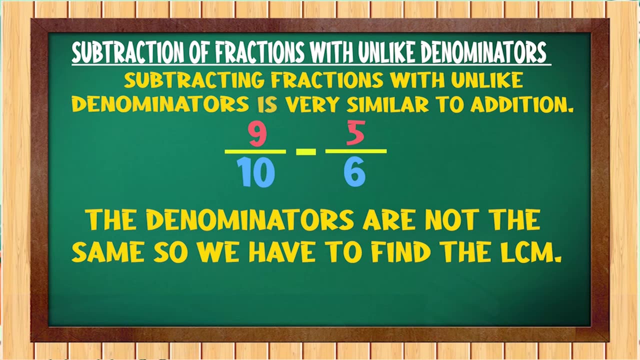 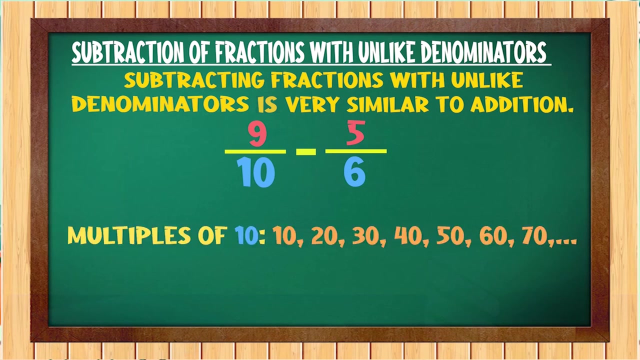 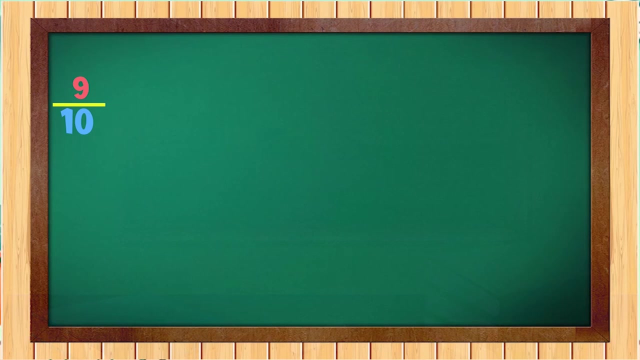 For example, if we were asked to find the answer for 9 10ths subtract 5 6ths, the denominators of those two fractions are not the same. So we have to find the lowest common multiple. So we're going to start off by listing the multiples of 10, which are 10, 20, 30, 40, 50, 60, 70. We're going to stop at 70, but we can go on. We will list the multiples of 6, which are 6, 12, 18, 24, 30, 36, 42. Now looking at the multiples of 10 and 6, we can see that the lowest common multiple is 30. Now that we would have identified the LCM for 6 and 10, which is 30, we can rewrite each fraction to its equivalent fraction with a denominator that is equal to 30. Okay? So to do this, we're going to split the fractions up. Let's look at the first fraction, which is 9 10ths. We're going to convert that fraction. Okay. To convert, we divide the denominator by the LCM.